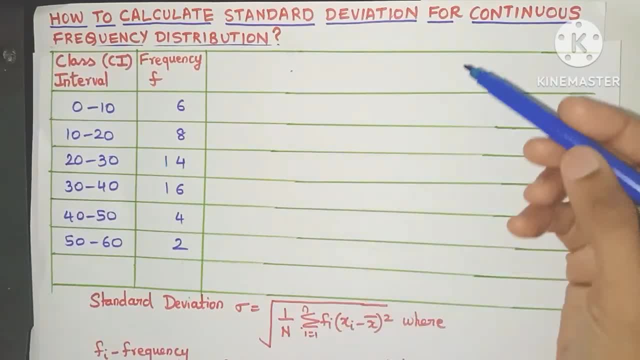 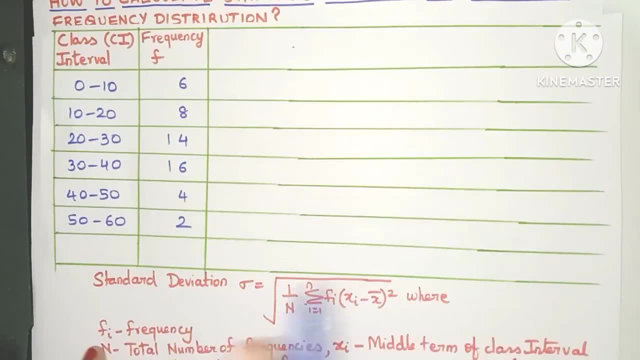 Hello everyone. today let's learn how to find the standard deviation for continuous frequency distribution. So here is the class interval column and this is the frequency column. Now this is the formula for standard deviation, but before we can use this, we need to find certain 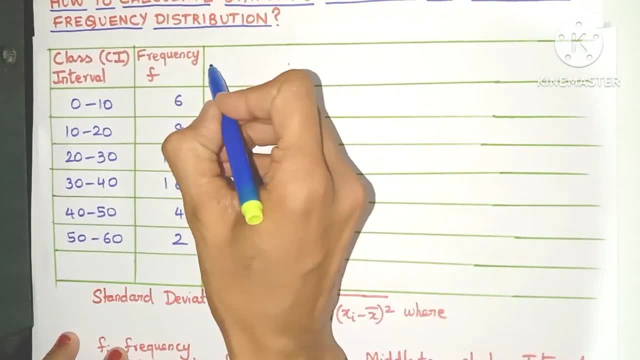 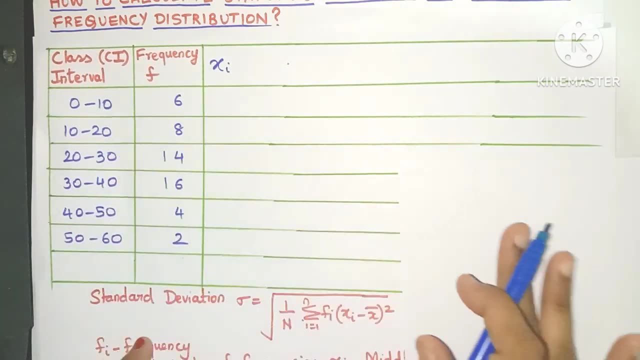 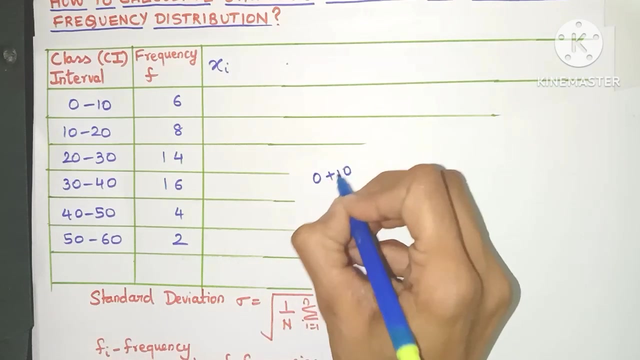 values. So for that let's create a new column, known as the xi column. Now, what is this xi? Now, it is nothing but the middle term of each class interval. So how do you find that is Just need to add the upper limit and lower limit and divide it by 2.. So 0 plus 10 divided by 2. 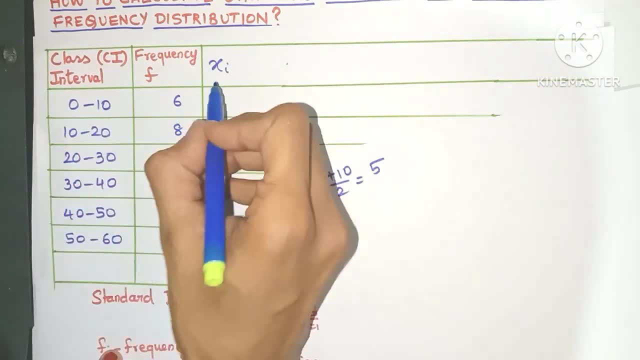 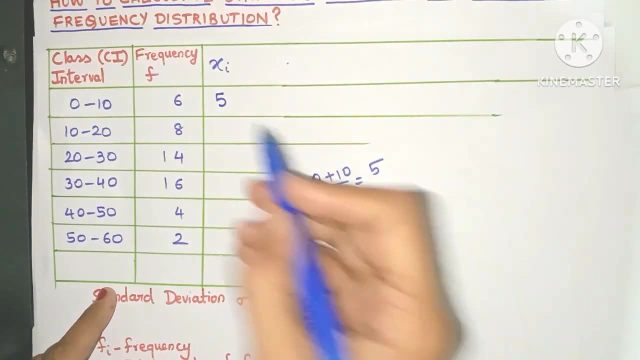 which is nothing but 5, and that is the xi value for the first class interval. friends, It's very easy. Now, that way, here you will see 10 plus 20,, 30,, 30 divided by 2, which is, yes, 15.. So this way, 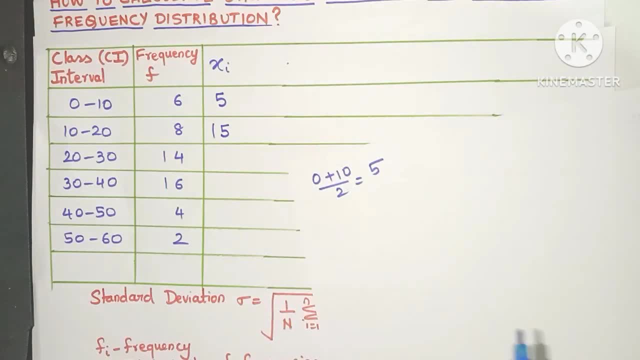 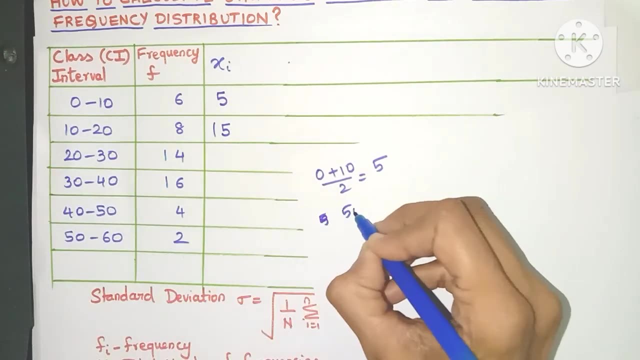 you can get all the xi values, but there is an easier way. What you need to do is just find the class size. So let's take this class interval. What is it? 40 to 50. So just subtract the upper limit and the lower limit, So we'll get 10. that is the class size. Now you 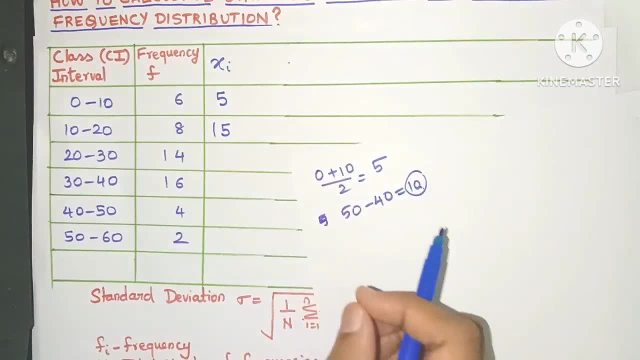 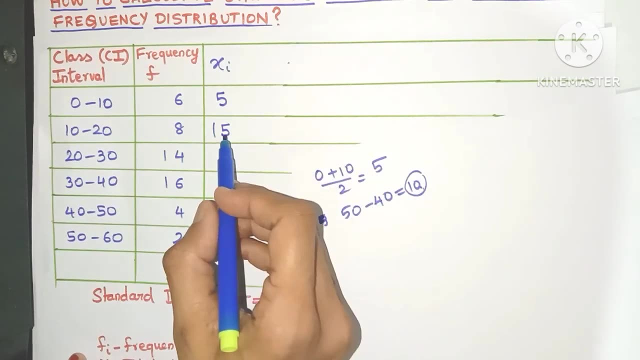 just need to add this class size to the first xi value, So 5 plus 10, which is 15.. So that way also, you will easily get the xi value. So what do we do now? You just need to add 10 to this 15. You'll. 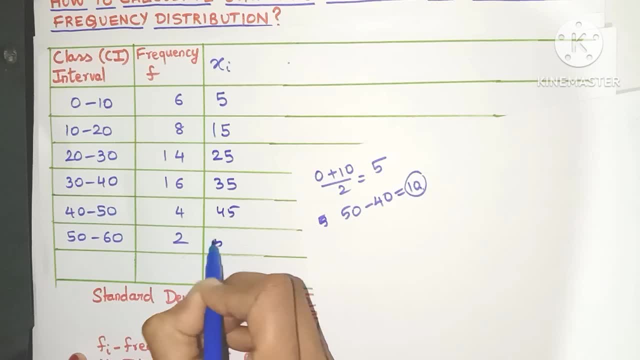 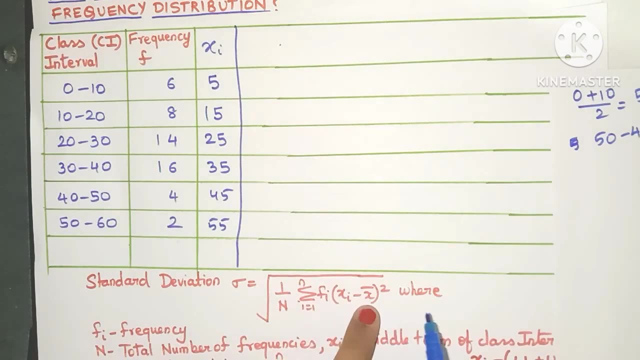 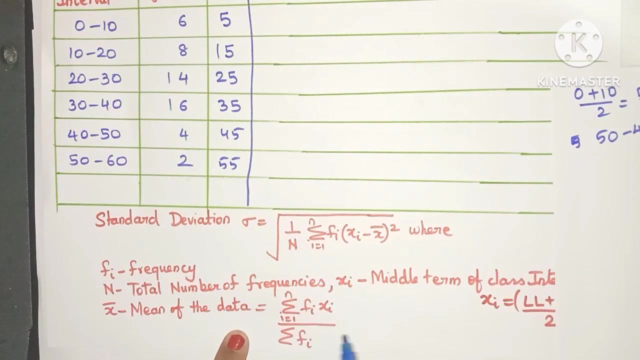 get 25,, 35,, 45 and 55 friends. So that's how you get the xi value. So we have got the xi values which we will need in the formula. Now. there is also x bar, which is nothing but mean of the entire data. The formula is sigma, fi, xi divided by sigma. 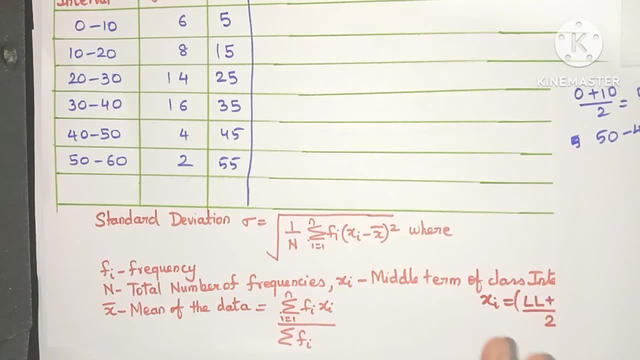 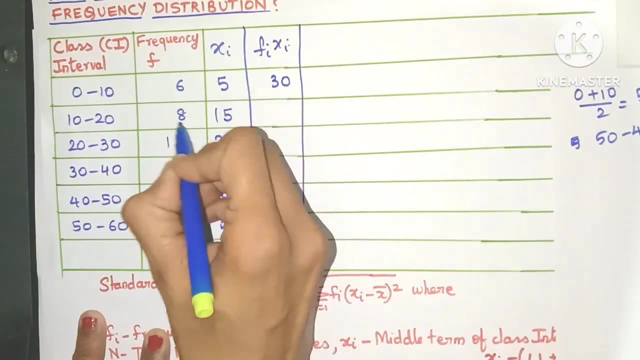 fi. Now, what is sigma? Yes, it's a greek symbol which means summation. So let's multiply fi and xi. Let's create the next column. Six fives are 30.. 8 into 15,, 120.. Now, while you're writing the, 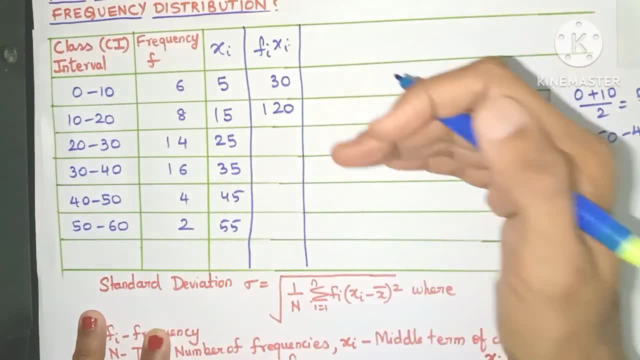 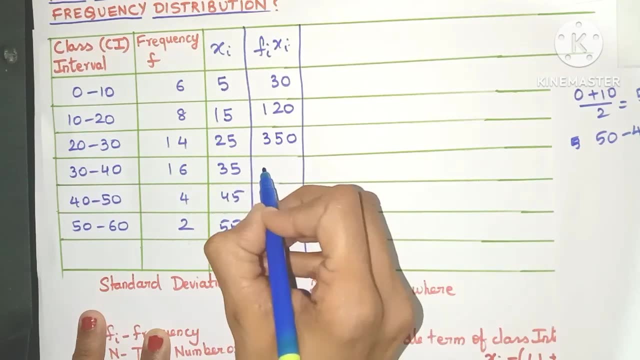 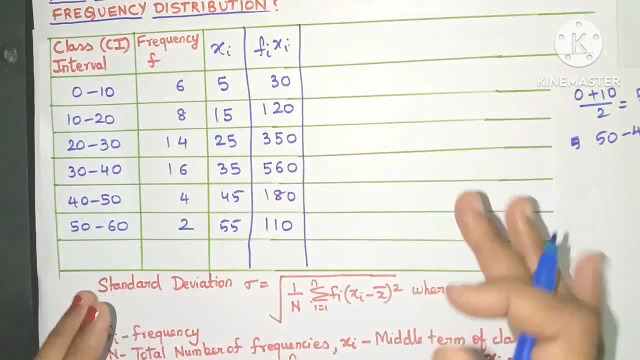 numbers. make sure to write the digits one below the other so that it will be easy when you're adding it. Now I've already done the calculations before, so I'll just copy the answers. You'll get 350.. This will be 560, 180 and 110.. So these are all the fi xi values, but we 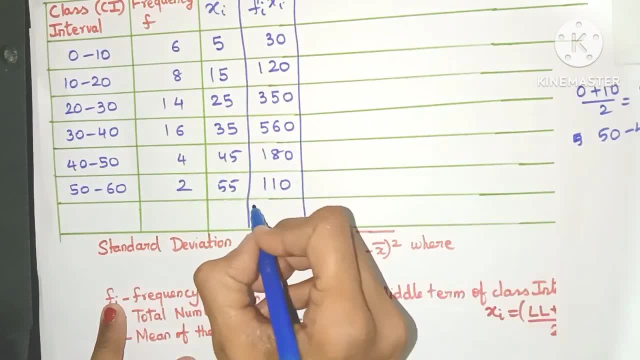 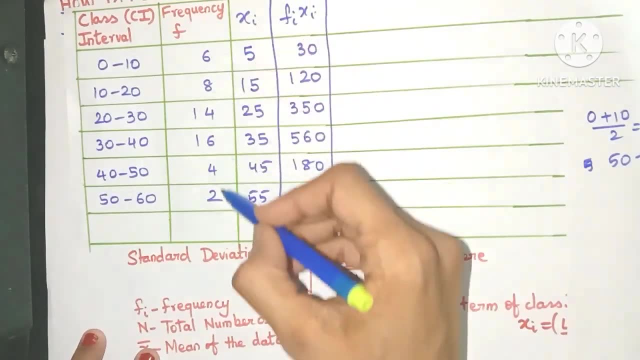 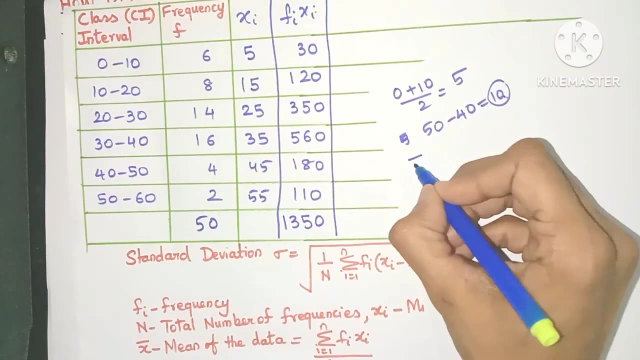 need to find their summation. So just need to add all of this. You'll get the answer as 1350.. Again, what is in the denominator Sigma fi? So let's quickly find the total frequencies. Yes, it comes to 50.. So now we can easily find the mean of this data. 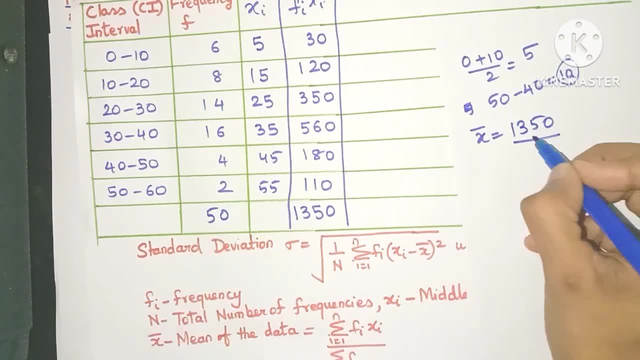 Sigma fi xi, which is 1350, divided by sigma fi, which is 50. So 00 gets cancelled. Yes, this will go in fi's table. Yes, so the mean is going to be 27.. Now this mean has to be subtracted from each xi. 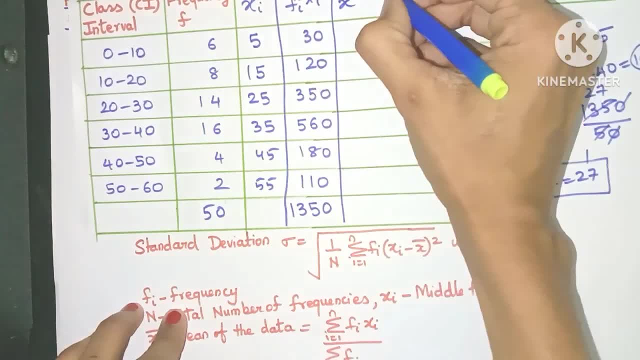 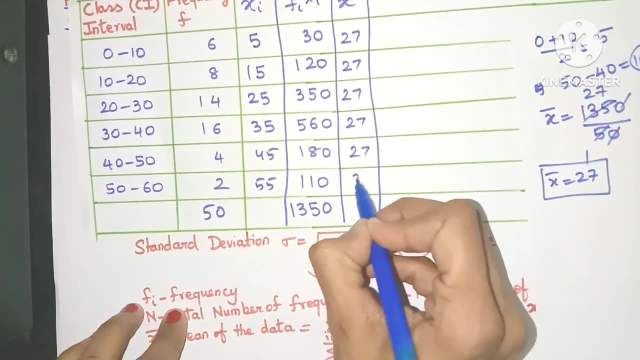 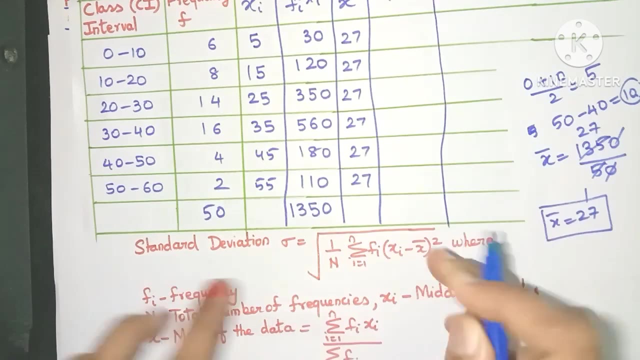 value friends. So what we will do is we will create a new column for the mean. Just need to copy the mean that we calculated for each class interval. Okay, like this. and now the next column we'll make is xi minus x bar. So just by looking at the formula, you will come to know what will be. 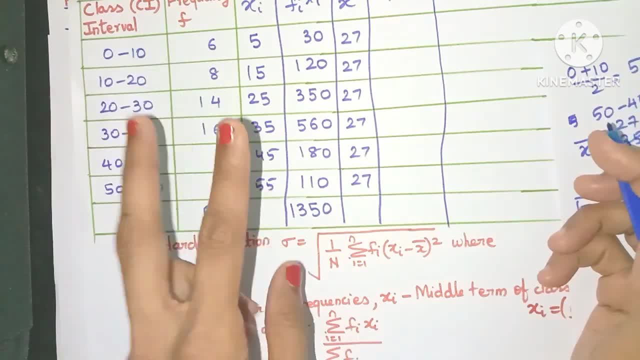 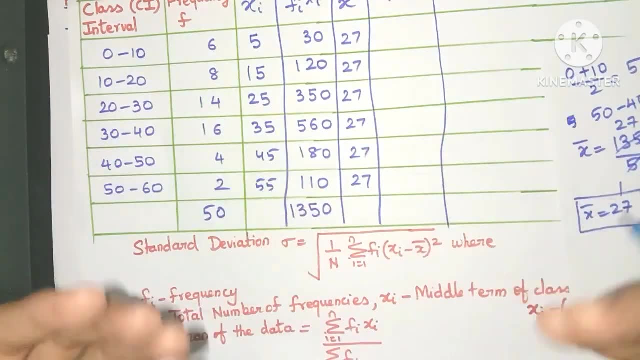 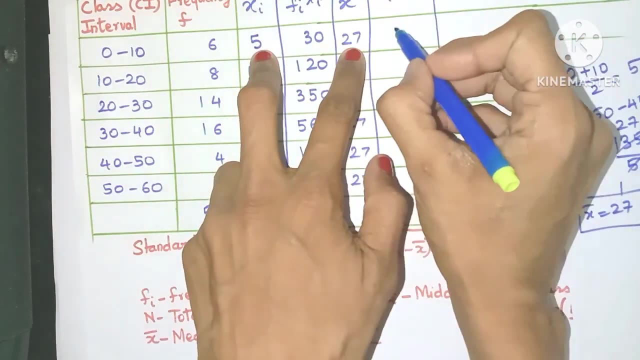 the next column that you need to form, So xi minus x bar. Let's keep the fingers on the columns that we want, because otherwise, since there are so many columns, you can easily get confused and may choose the wrong column. So just use your fingers to help you out. So you need to do 5 minus 27 friends. So 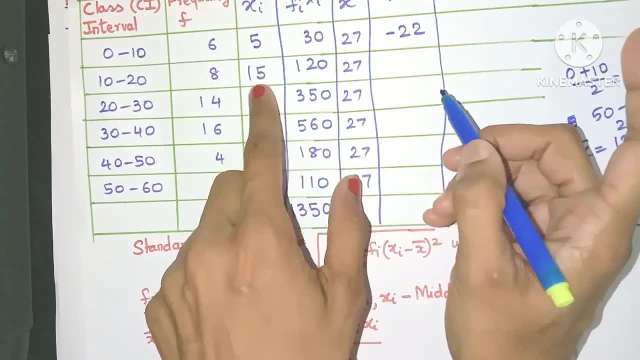 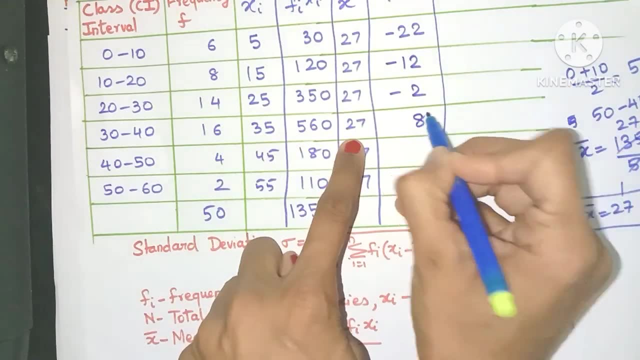 what is it? Yes, minus 22.. Remember there's a minus sign. Same way, 15 minus 27.. So you need to do 5 minus 27 minus 12.. Here it will be minus 2.. 35 minus 27, 8. This will be 18 and, yes, this will be. 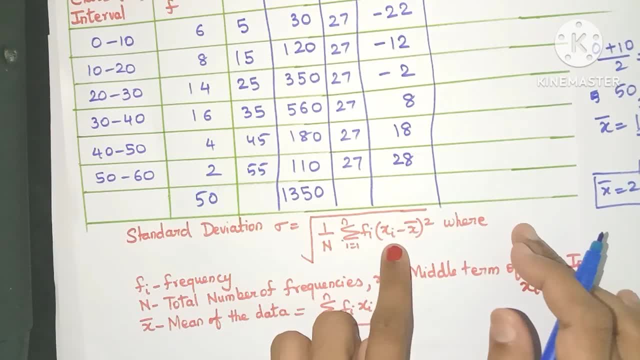 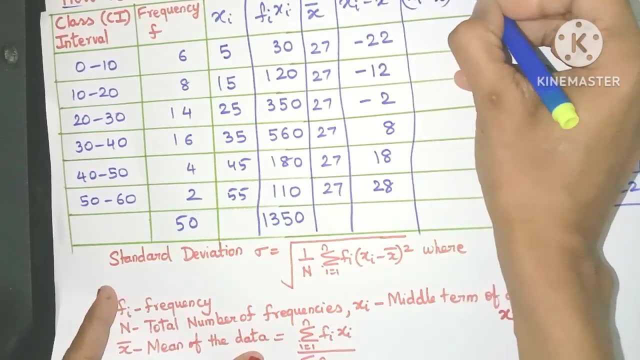 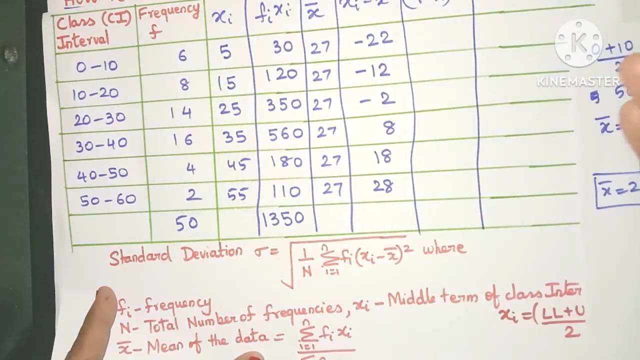 28.. Now what do we need to do next? That's right, We need to square this: See xi minus x, bar the whole square. So that will be our next column. Just need to keep looking at the formula for the next column. So just need to square this. So when you square, automatically the minus sign goes off. 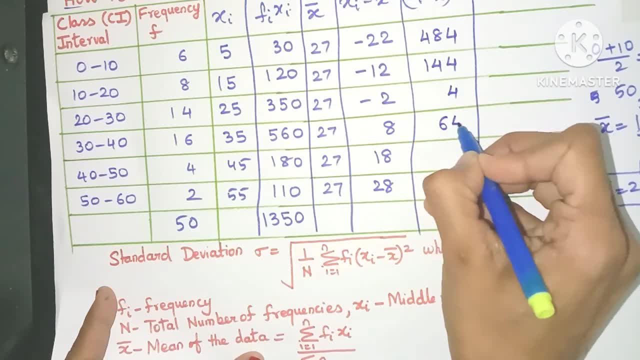 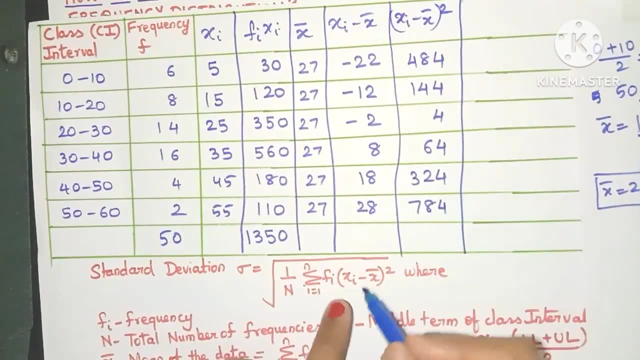 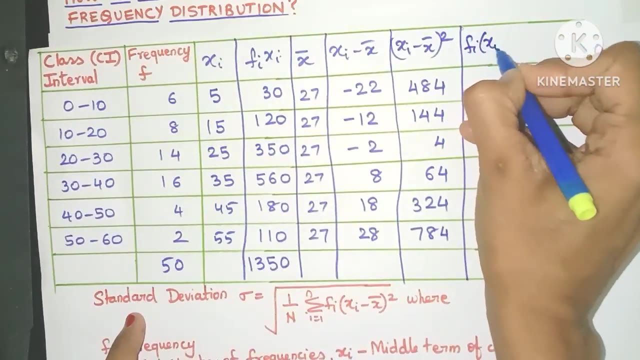 Okay, you can fill up all these rows over here: 64,, 324 and 784 friends, So this column is also completed. Again, if we look at the formula, we need to multiply this term with the fi value. So that will be the next column over here. So which are the columns to be chosen? This frequency column? 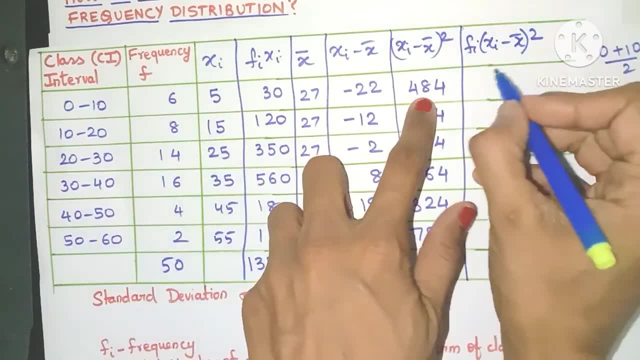 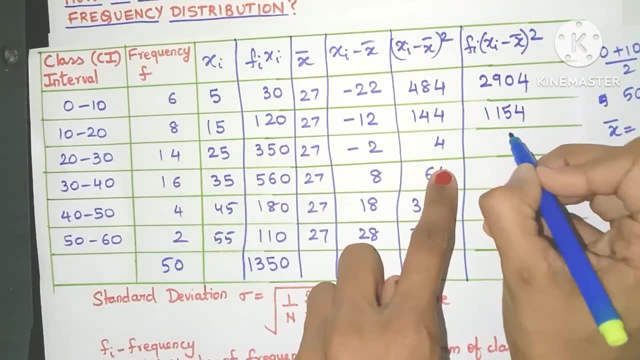 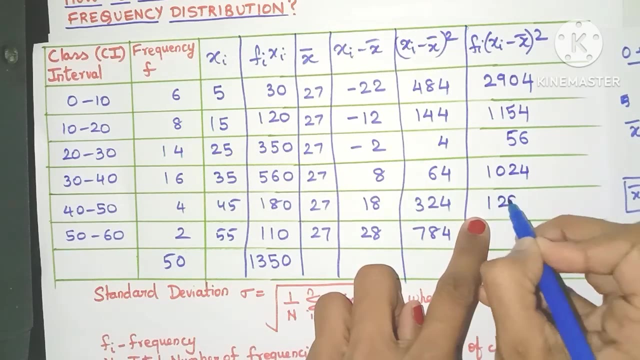 and this column over here. So 6 into 484.. I've already done the calculation, friends, So I'm just as it is. Please use ample rough space to do the calculation so that you get the answers correct. So this will be 1024.. This will be 1296, and here 2 into 784 will be 1568.. Now, what do we need to? 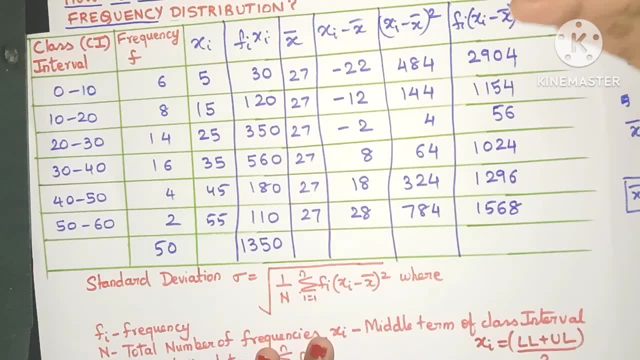 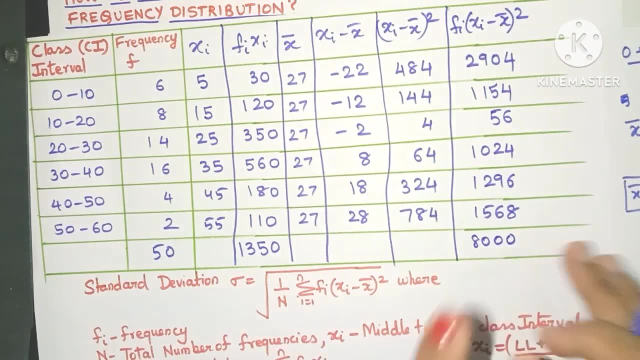 do Again. look at the formula. We need to do the sigma. That is the summation. So add up all these values very carefully. You will get 8000 as the answer. Now what do we need to do? We have already. 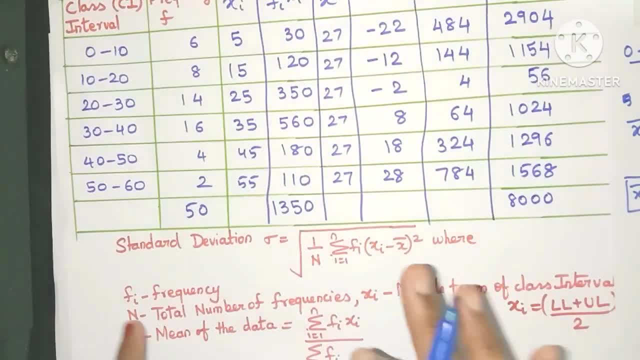 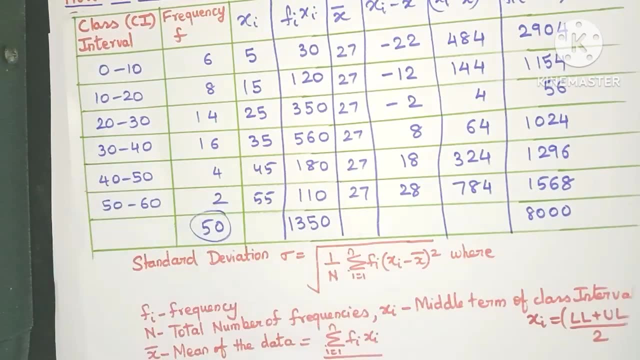 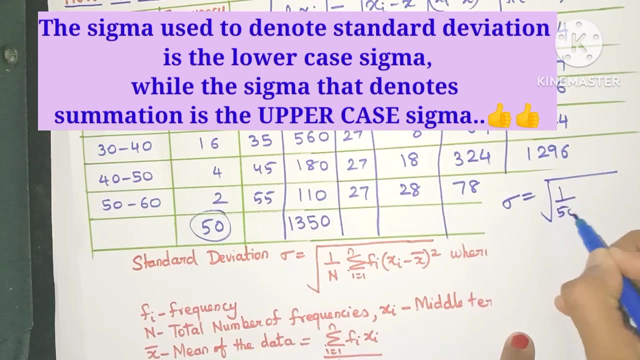 got this sigma value. Now, what is this n? Yes, n is nothing but the total number of frequencies. but we have already calculated that over here, See 50.. So it's time to do substitution. So sigma, that is standard deviation, is square root of 1 upon n, that is 1 upon 50 into this whole thing is 8000.. 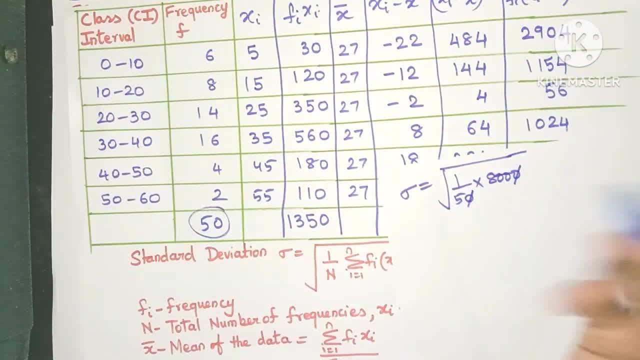 So I hope you're clear till here. Now just calculation part is remaining. So I'll get 800 by 5, which is yes, it will go in the 5's table. Yes, I will get root of 180.. Now, this is the standard deviation. 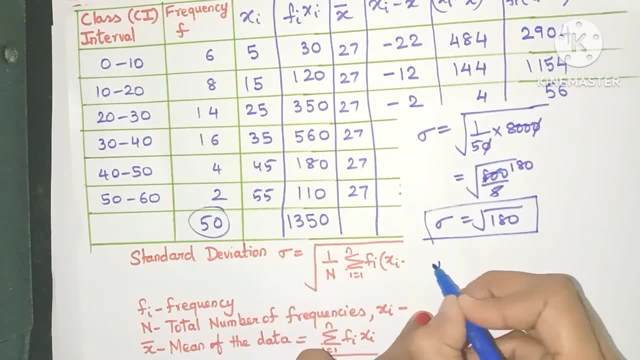 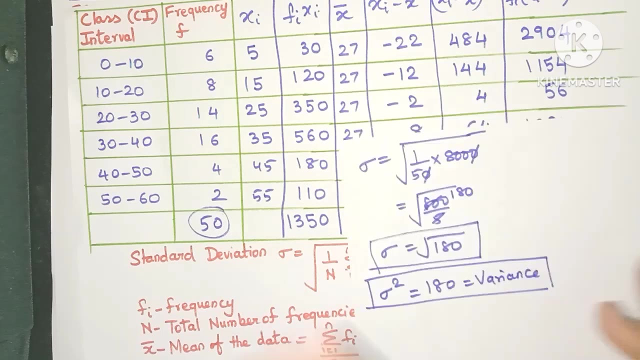 Now, if they are asking for the variance, Remember friends, variance is sigma square, So sigma square, or the variance is 180 and that's how you will get the variance. However, here they have asked the standard deviation. So let's go ahead and find the square root of 180.. You can. 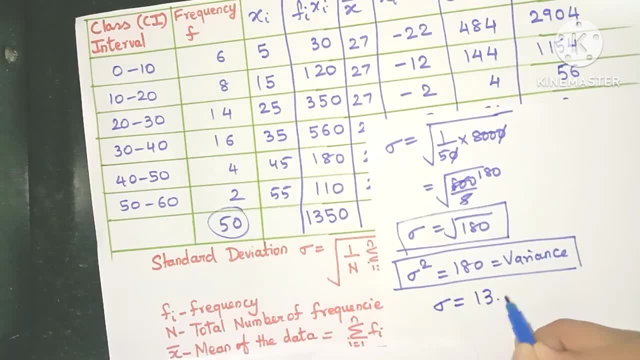 use the long division method, So sigma is going to be 13.416.. This is how you find the standard deviation for continuous frequency distribution. So, friends, I hope that you found this video useful. If so, please do like and share the video. Consider subscribing. 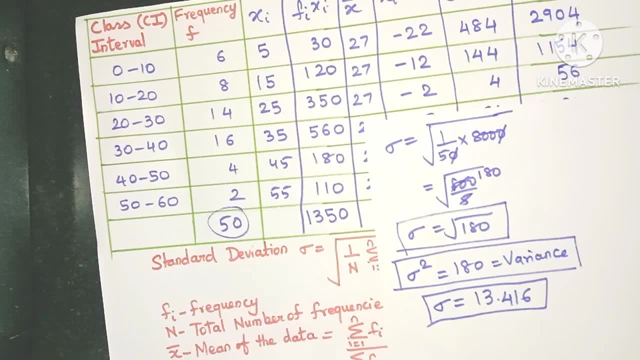 to enjoy math and please leave your comments in the comment section below. So till we meet again. take care.